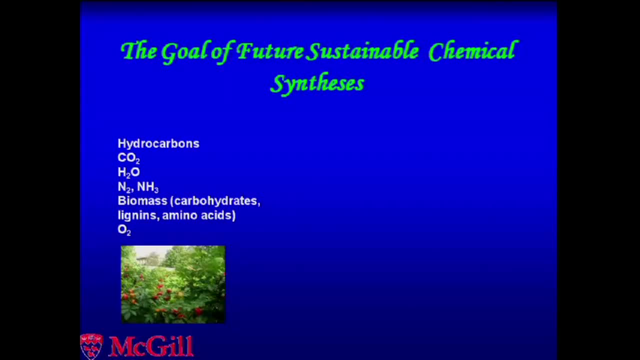 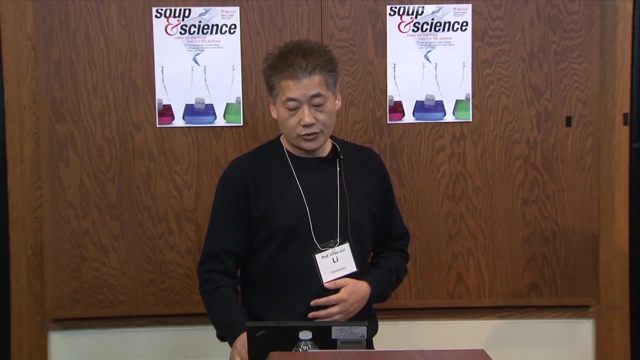 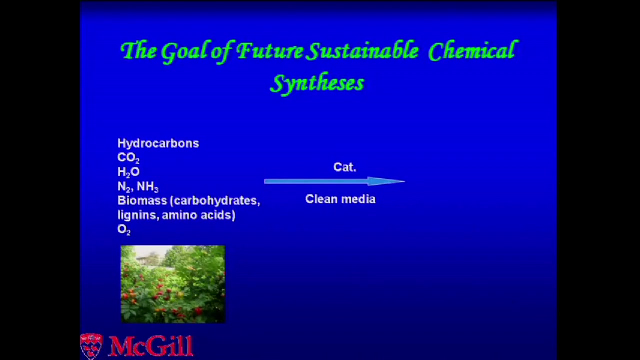 basically, such as the hydrocarbon, CO2, lignans, cellulose, as you can find, and based on renewable basis and through very simple reactions, by inventing a very simple reactions through catalysis in clean solvent such as water and turn them into useful chemical products directly. Of course, this is a very wishful thinking, But really what? 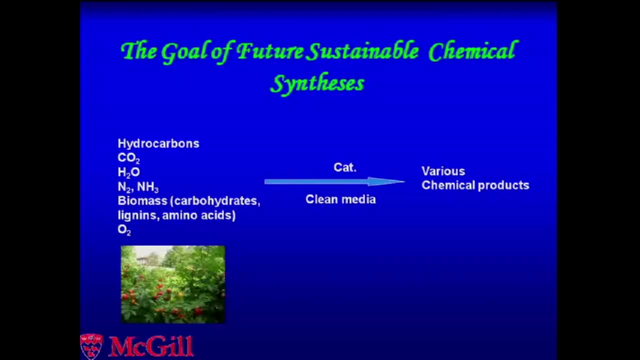 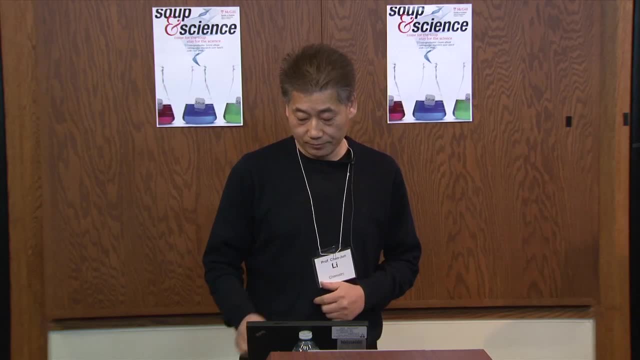 we have to do. at the end, after many, many years, we would like to have some new reactions, some new tools available, new science, new chemical science available so that we can complete this, And so, of course, we need to explore new reactions. 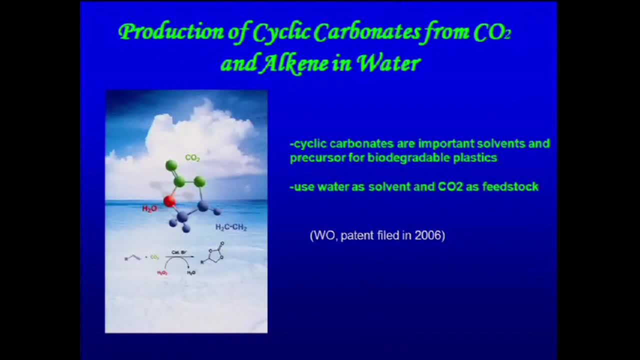 That's what we're trying to do in our group And just give you a very quickly two example- And this is a patent actually by McGill- where we take carbon dioxide alkene in water, sort of very simple catalyst such as bromine, with hydrogen peroxide and air. 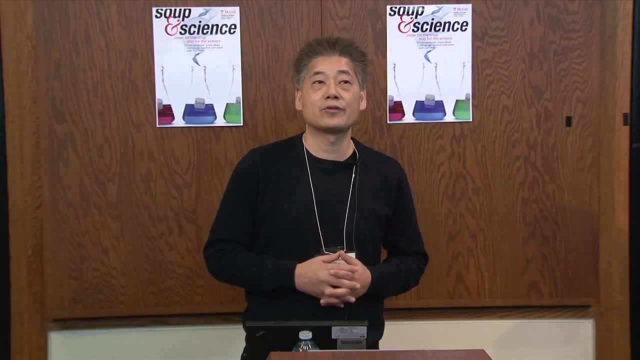 We can turn them into cyclic carbonate, which itself is a very useful solvent- already It's called the greener solvent- And furthermore, industrially you can polymerize these into biodegradable plastic, where, of course, when you're three in nature, 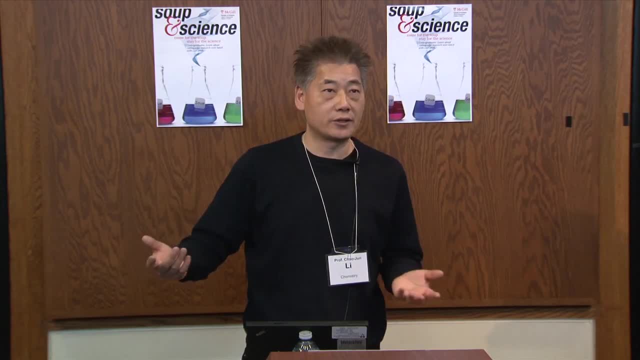 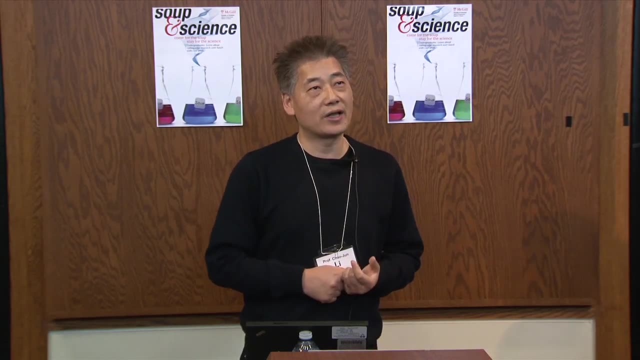 will decompose very quickly, Unlike the current plastic will take about a hundred years to degrade. The another example: of course, for chemists sitting here, the most important reaction in chemistry is the greenhouse reaction. but you have, they are very sensitive. 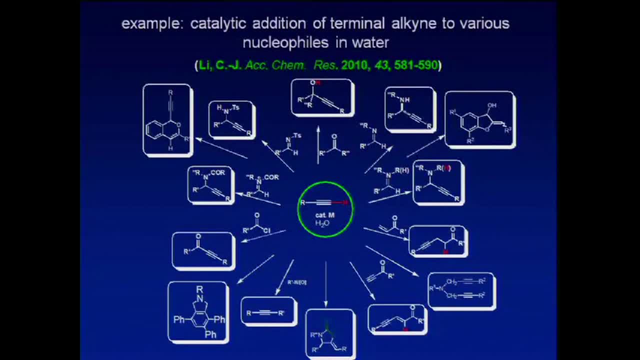 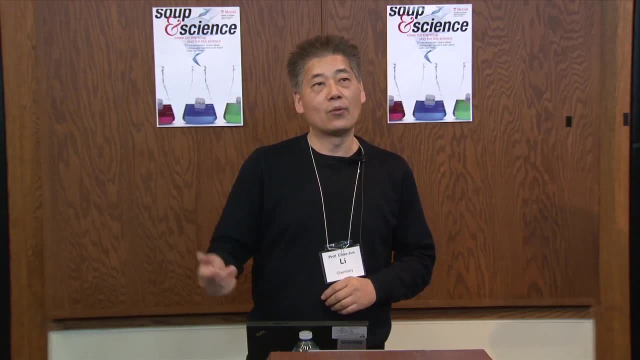 and you have to protect on nitrogen and use an hydrosolvent And, furthermore, you have to synthesize them. So we developed a process where you can take the simple alkyne or alkene and the water and the fungal growth in the water. 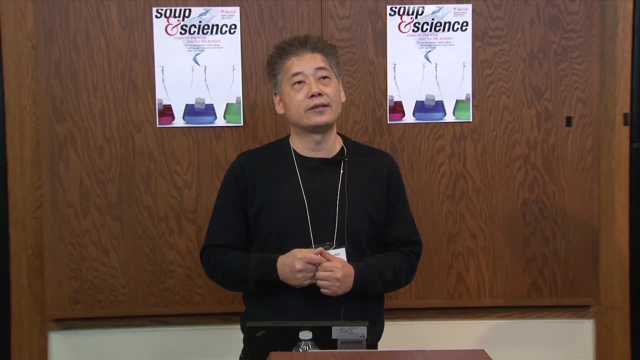 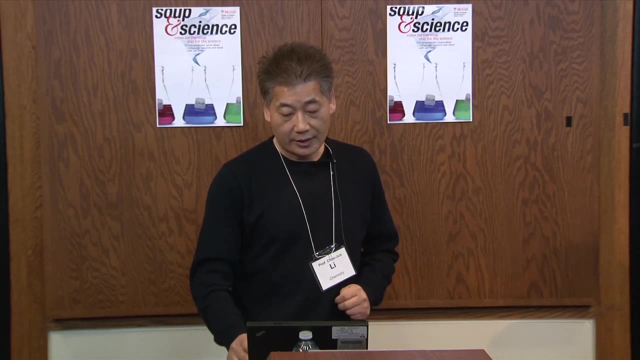 by using a simple catalyst stirring water and mostly in air, you turn them into product directly. There's virtually no waste left behind. So that's what we developed, And so finally, in the end, what we hope to do is through green chemistry, research. 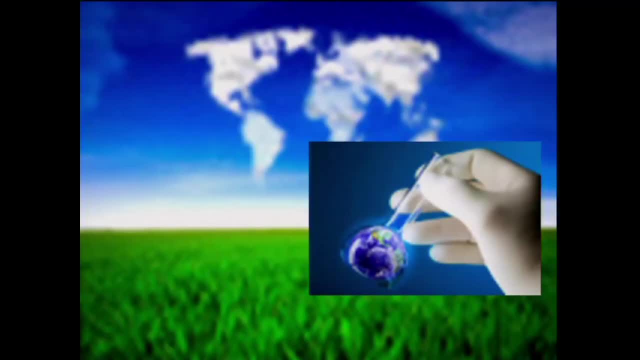 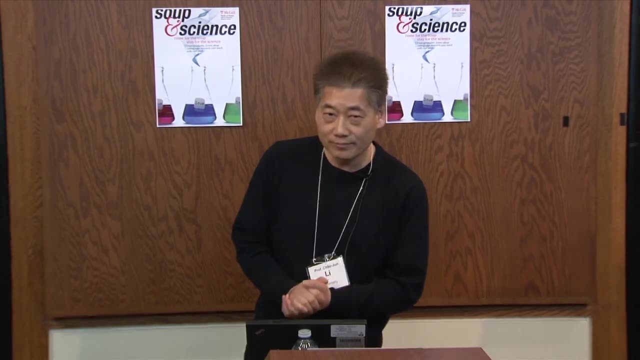 we will have a sustainable society and both have a healthy environment as well a clean the chemical manufacturer industry. Thank you,